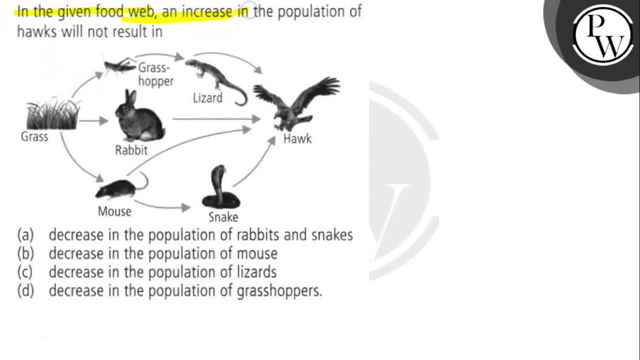 Hello virtual. let's read the question. The question says: here, in a given food web, an increase in the population of hawks will not result in. So, in the given food here, an increase in the population of the hawk will not result in, So what will be occur? So this is the food web representing the feeding relationship with the ecosystem. This is the food web. 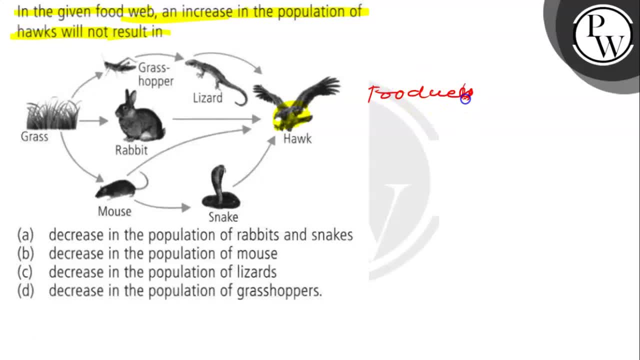 That is food web. That is different kind of food chain connected with each other and forming a web like structure. This is known as the food web and also including many interconnected food chain. It is in the given food web. The hawk is the. this is the. this is the. this is the top consumer. This is the top consumer. that feed measure upon the lizard. This is measured upon the lizard, rabbit and the snake. 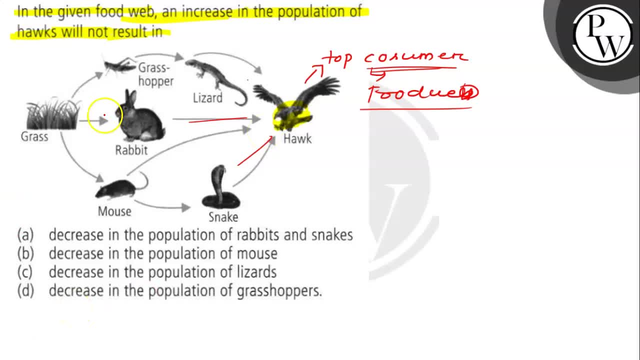 So this is. so this is known as the top consumer and in unavailability of this animal, of this, that is enough. this top consumer, The hawk, fed upon the mouse and grasshopper. So when there will be absence of lizard rabbits and snake, So they, they eat the grasshoppers, or they eat them, or mouse, They eat the mouse, or grasshoppers or rabbit, So easily available. So this, this will decrease the population of the lizard rabbit and the mouses. So that means that means the reduction of the 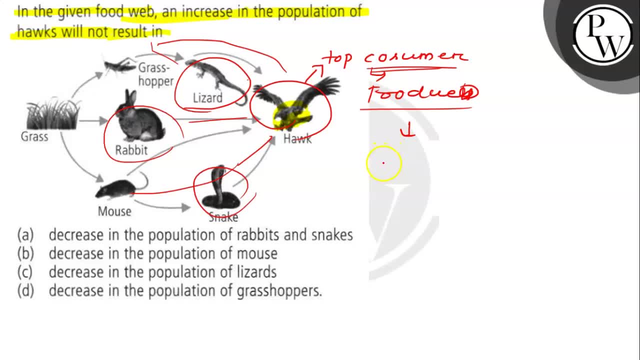 So the reduction, reduction of the population decreases, decrease in the population of the rabbit. So in in this, in this question, that is, increase in the population of the hawk will not result in. So when there will be population increase in the hawk, this will, this will result in. 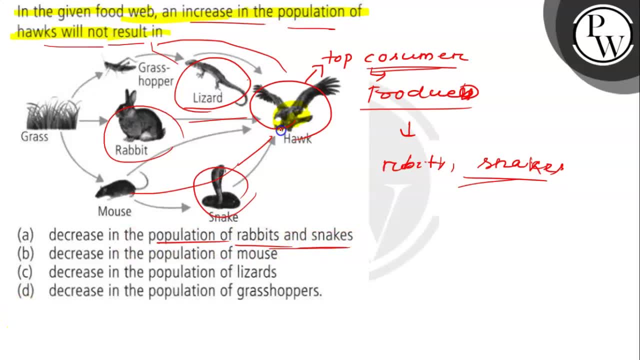